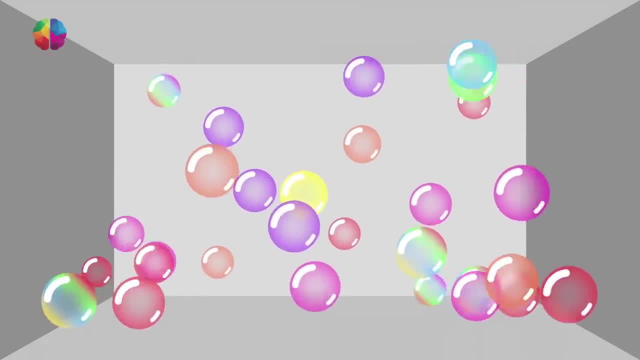 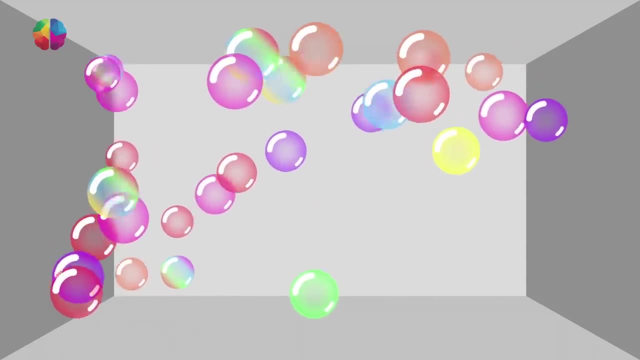 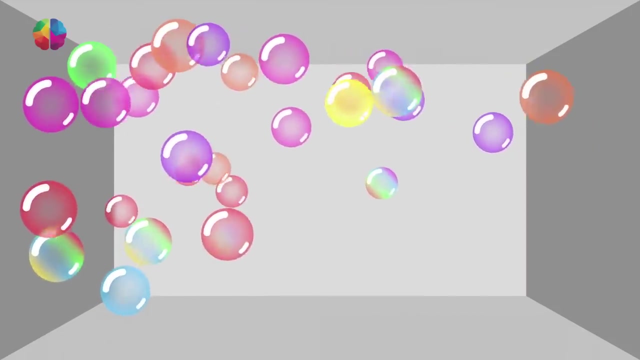 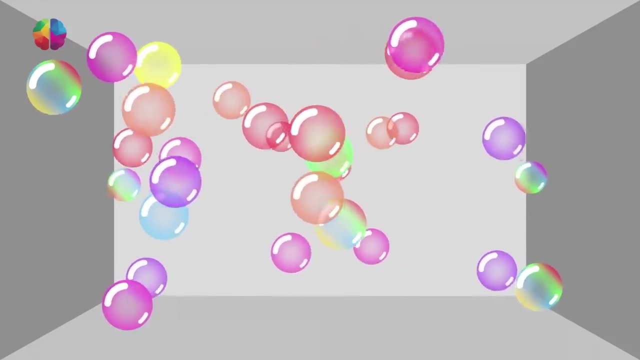 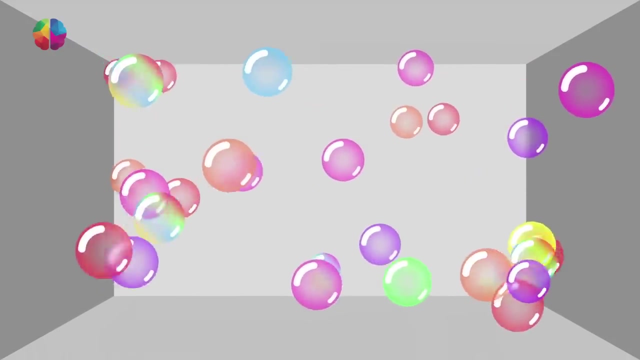 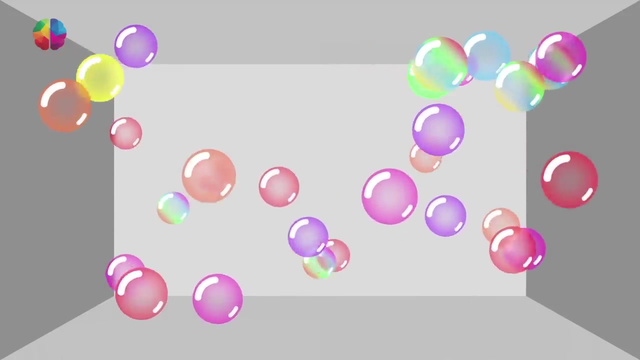 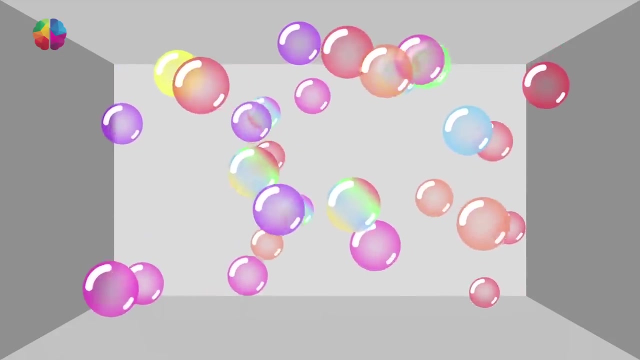 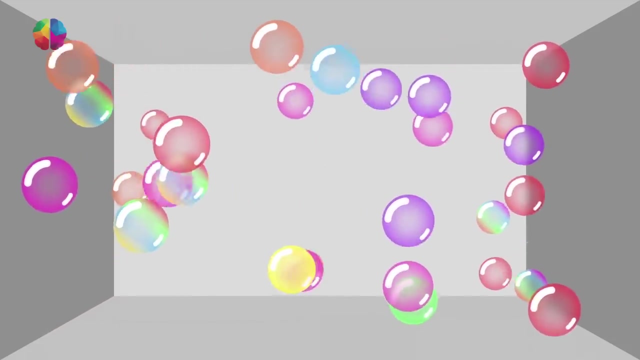 it goes with your eyes. Don't be tempted to look at any other bubble. Stay with the yellow one. Pay close attention to it. Now look at the yellow bubble. Don't be tempted to look at the blue bubble. Follow it closely, Keep looking. Some of them might start to pop to try and distract you, but don't let them. 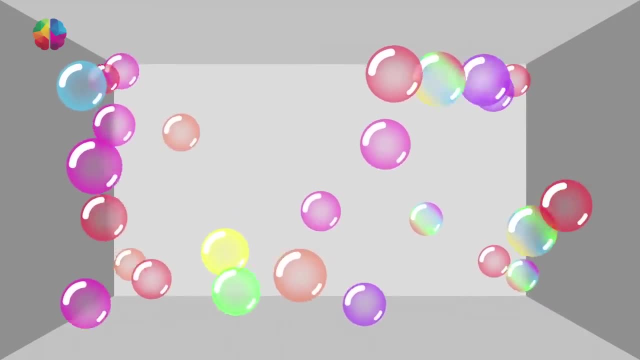 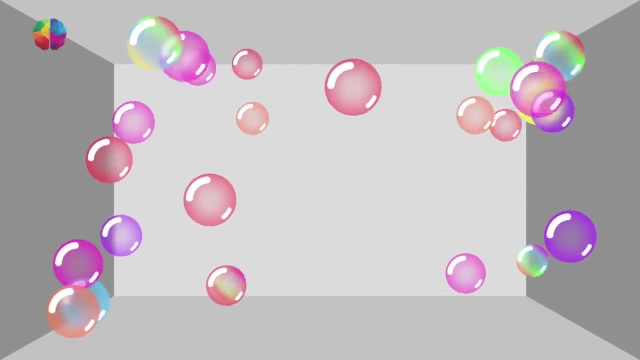 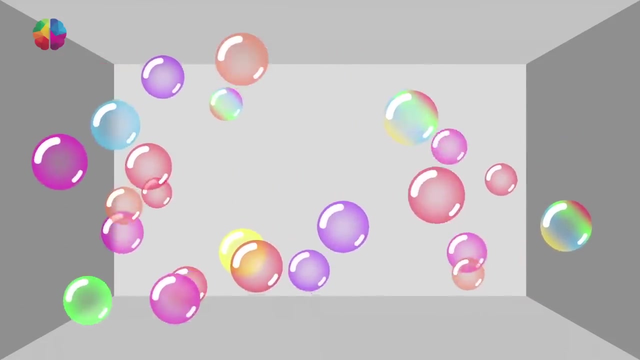 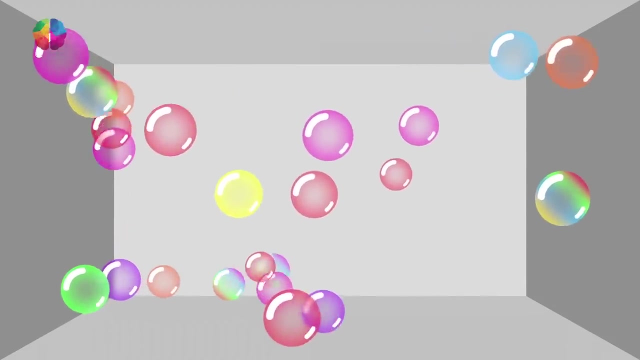 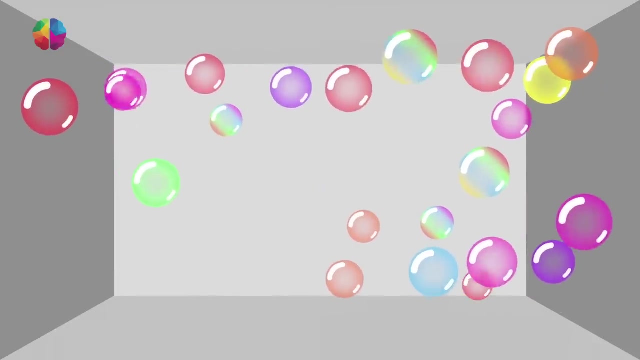 Now switch to the green one. Pay attention to it. This means only think about this one thing. Keep track of it, even if it goes behind another bubble. Keep the этоtique careful. Try not to make her see anything big or small. 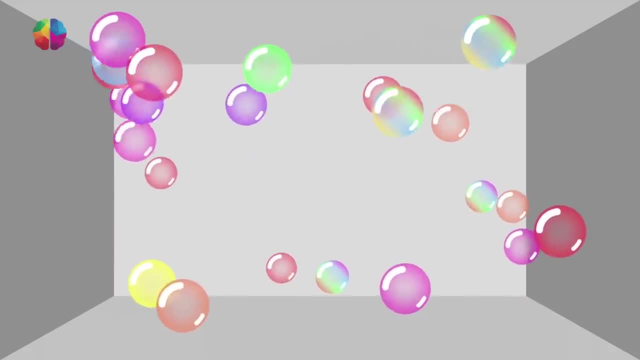 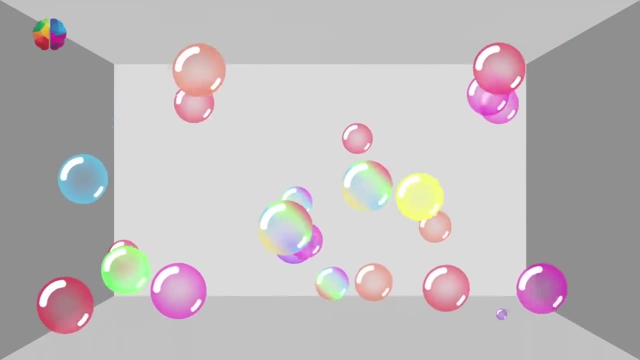 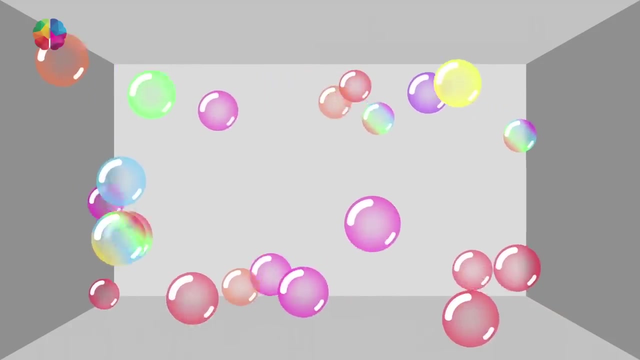 It doesn't happen. Keep trying to look at the blue bubble by holding the second heel of your Дuh own. Now look for the smallest bubble. Your eyes will have to scan over the whole screen to spot it. Don't shout out which one it is. stay silent. 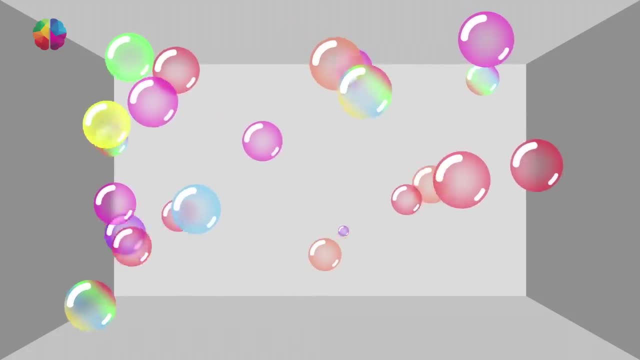 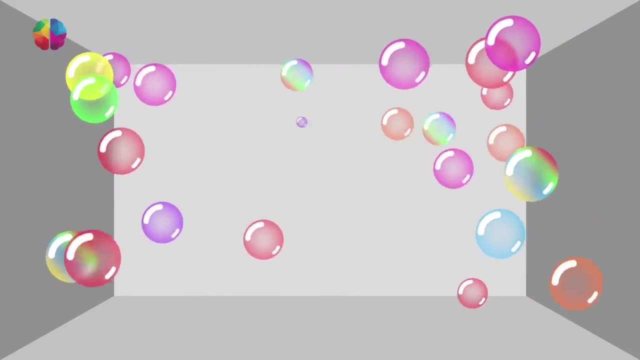 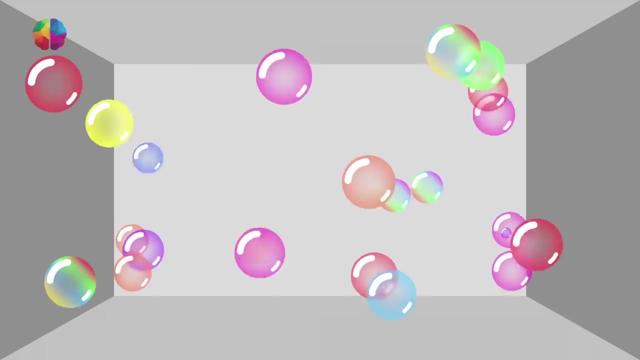 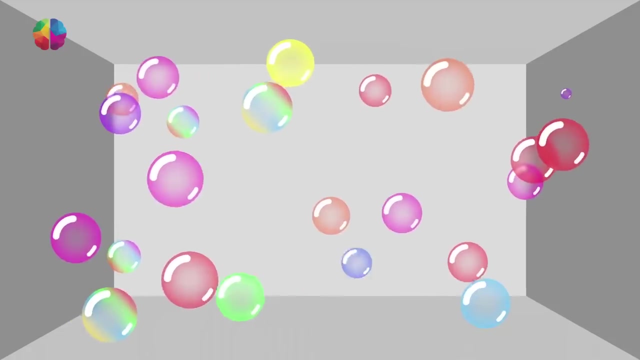 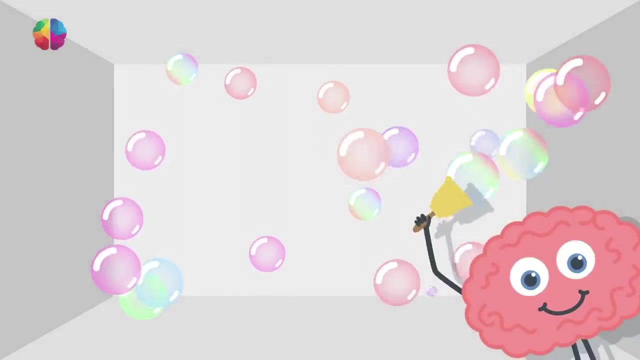 Now pay attention to the fastest bubble. Well done, Now you've exercised your focusing skills, you can put these into practice in your lessons.